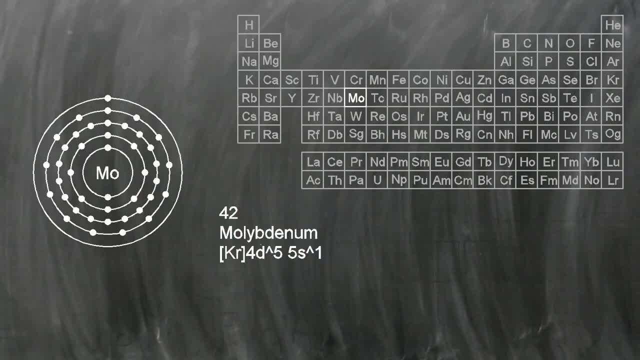 Neobium, Molybdenum, Technetium, Ruthenium, Rhodium, Palladium, Silver, Cadmium, Indium, Tin, Antimony, Tellurium, Iodine, Xenon, Cesium, Barium, Lanthanum, Cerium, Praseodium. 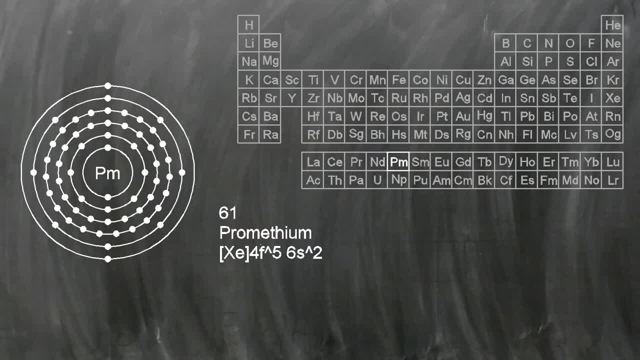 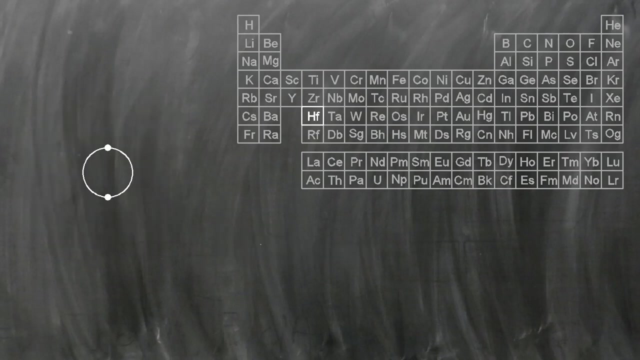 Neodymium, Promethium, Sumerium Europium, Gadolinium, Terbium, Dysprosium, Holmium, Iterbium, Thulium, Iterbium, Lutetium, Hafnium, Tantalum, Tungsten, Rhenium, Osmium, Iridium. 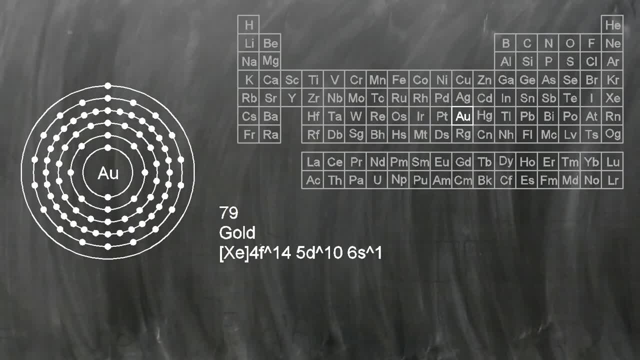 Platinum, Gold, Mercury, Thallium, Lead, Bismuth, Polonium, Astatine, Radon, Francium, Radium, Acneum, Thorium, Protactinium, Titanium, Uranium, Neptunium, Plutonium, Ameritium, Curium, Perkelium, Californium. 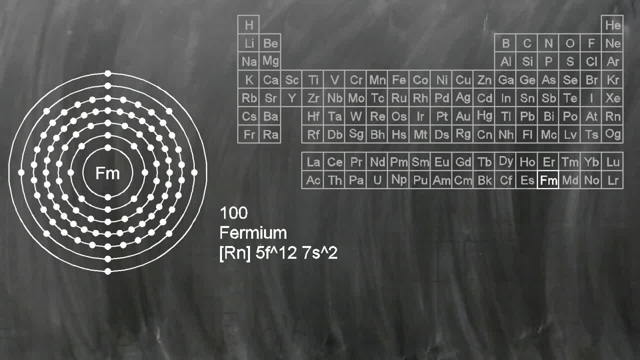